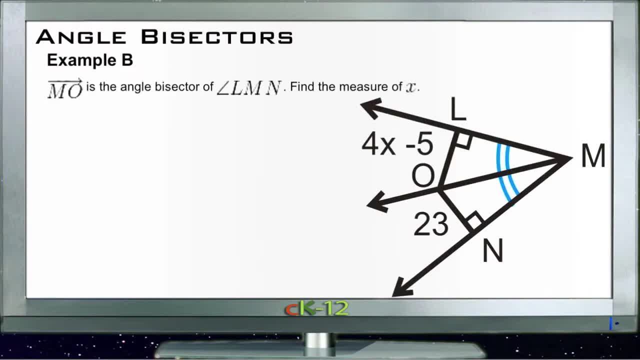 Okay, let's take a look at example two, or example B. Example B says: right, here is the angle bisector of l m n. So the angle bisector of l m n. that tells us that of course, these two angles here are the same And we need to find the measure. 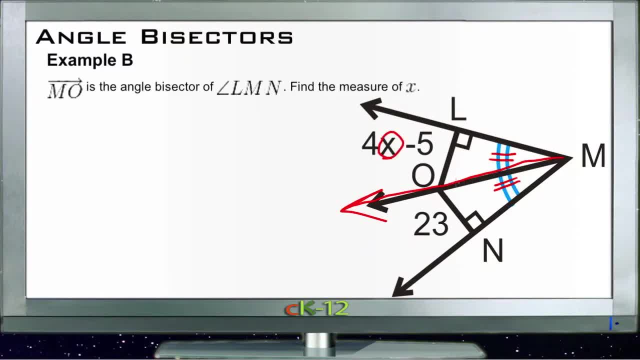 of x right here. Well, since this is the angle bisector that tells us that this line here is congruent to this line here, which means that 4x minus 5 is the same thing as 4x minus 23.. So we just need to solve for x. We'll add 5 to both sides. 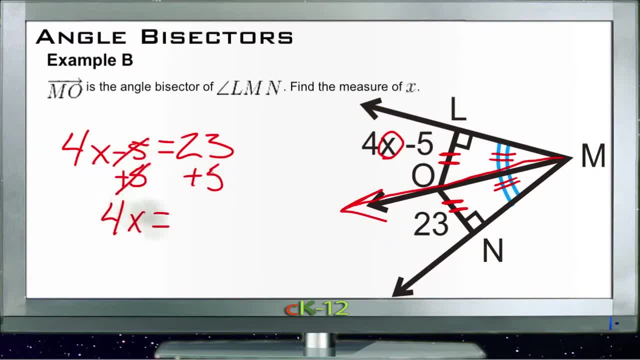 5s- cancel. We have 4x over here. 23 plus 5 is 28.. Divide both sides by 4.. 4s- cancel. We get x equals 28 divided by 4, which is 7.. So x. 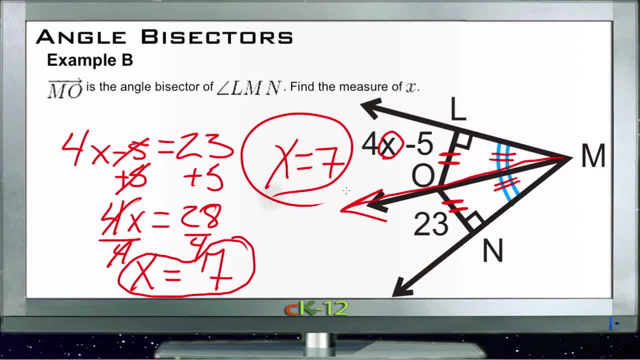 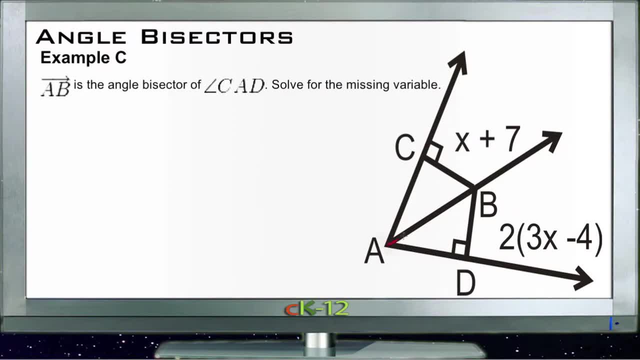 is seven. okay, example c: sample c says ray a- b: right here is the angle bisector for c a d. right here c a d and we need to solve for the missing variable. so in this case, solve for x. now, if this ray a- b is that angle bisector as we're told, then that means that c- b is congruent. 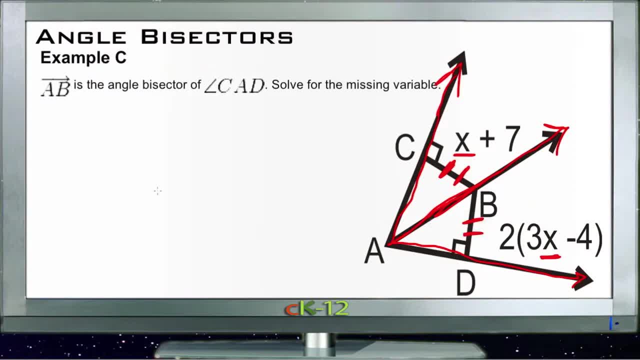 to b, d, as in the last example. so that tells us that x plus seven is equal to two times three x minus four. so now we just need to solve for x. so first we'll distribute that two, we get two times three x, that's 6x, and 2 times negative. 4 is negative. 8, is equal to x plus 7.. 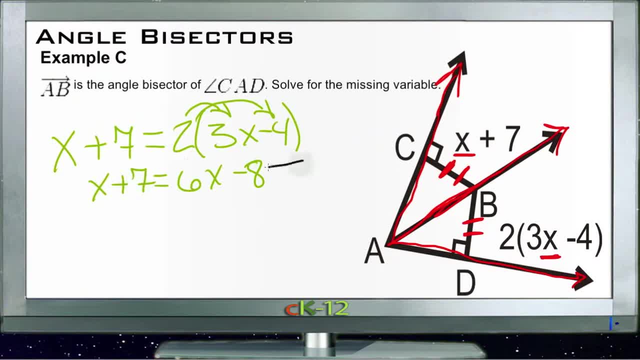 Now we have more x's on this side because we have 6x's over here and only 1x on the left side. so let's move the x's to the right-hand side, So we'll subtract x over here and that'll cancel and subtract x over here.